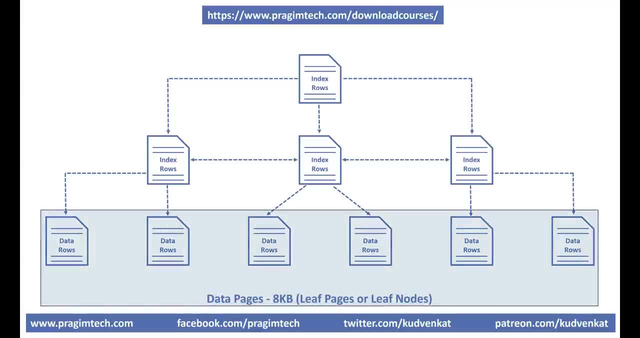 bottom of the tree are called data pages or leaf nodes of the tree, and it is these leaf nodes that contain our table data. The size of each data page is 8 kilobytes. This means the number of rows that are stored in each data page really depends on the size of each row. For our example, let's say: 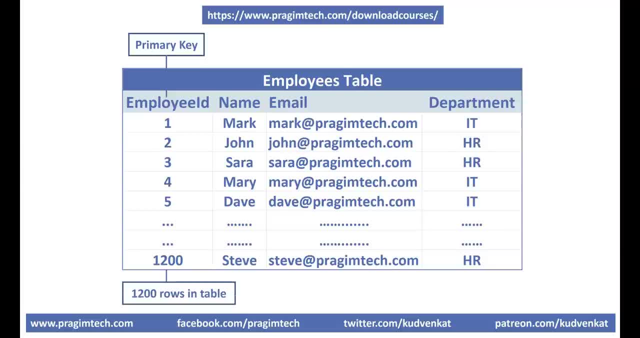 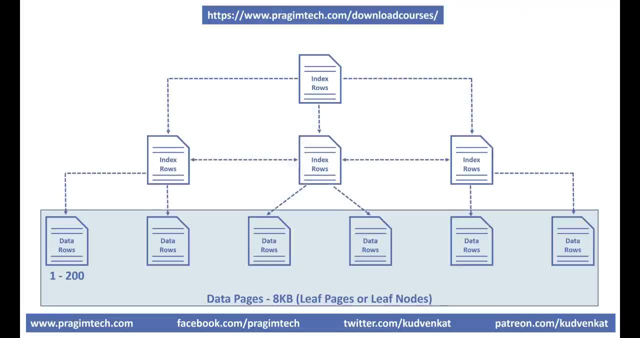 in this Employees table we have 1200 rows And let's assume in each data page we have 200 rows, But in reality, depending on the actual row size, we may have more or less rows. But for this example sake, let's assume each data page. 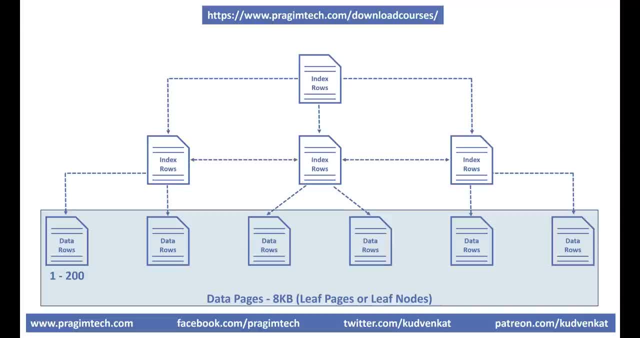 has 200 rows. Remember. the important point to keep in mind is the rows in these data pages are sorted by Employee ID column, because Employee ID is the primary key of our table and hence the clustered key. So in the first data page we have 1-200 rows, in the second 201-400,, in the third, 401-600,. 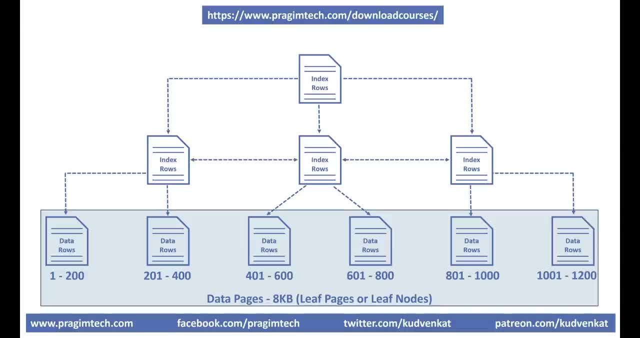 so on and so forth. The node at the top of the tree is called Root node. The nodes between the root node and the leaf nodes are called intermediate levels. They can be multiple intermediate levels. In our example we have just 1200 rows and to keep this example simple, 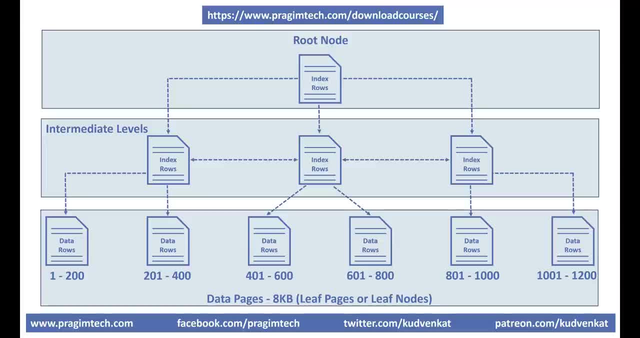 we need just 1 intermediate level, But in reality the number of intermediate levels depends on the number of rows you have in the underlying database table. The Root and the intermediate level nodes contains index rows and the leaf nodes, that is, nodes at the bottom of the tree, contain the actual data rows. 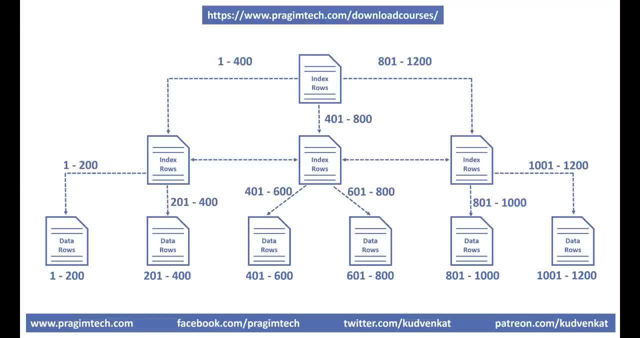 Each index row contains a key value, in our case Employee ID, and a pointer to either an intermediate level page or an actual data row. Note that in this example here we need to in the B-tree, or a data row in the leaf node. So the important point is this tree-like structure. 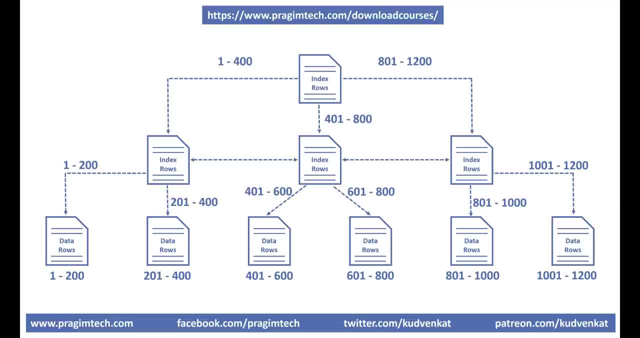 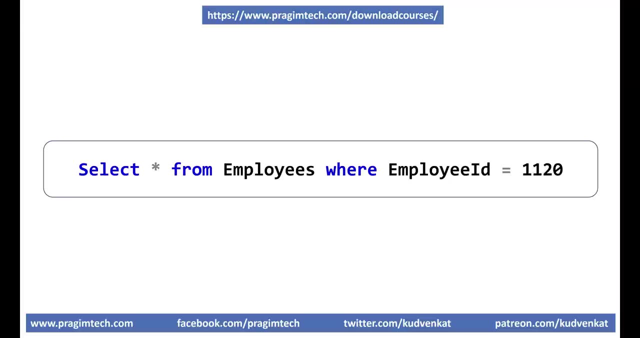 has a series of pointers that helps the database engine find the data quickly. For example, let's say we want to find employee row with employee id equals 1120.. So the query itself is very simple: Select star from employees where employee id equals 1120.. So the database engine starts at 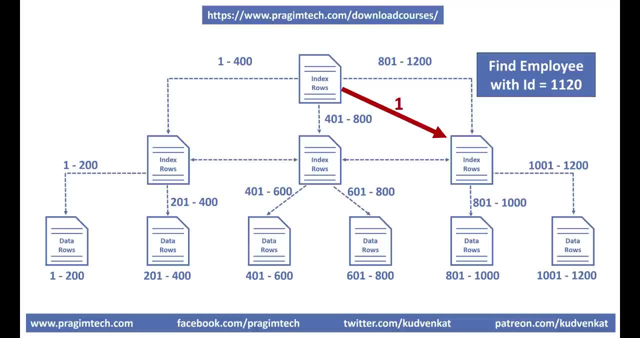 the root node and from there it picks the index node on the right, because the database engine knows it is this node that contains employee ids from 801 to 1200.. From there it picks the leaf node that is present on the extreme right, because employee data rows from 1001 to 1200. 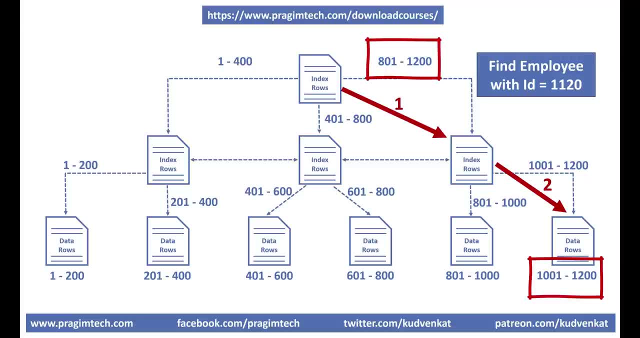 are present In this leaf node. the data rows in the leaf node are sorted by employee id, So it's easy for the database engine to find the employee row with id equals 1120.. Notice, in just three operations SQL server is able to find the data we are looking for. So the point is, if there, 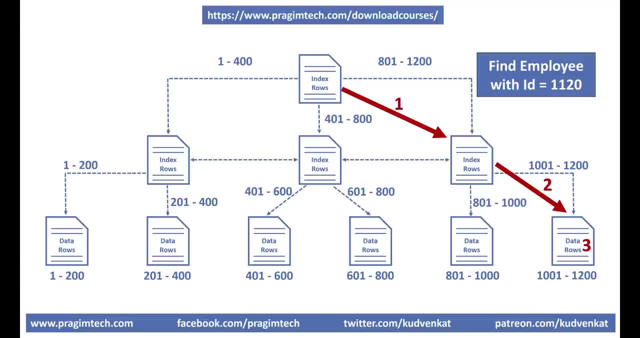 are thousands or even millions of records, SQL server can easily and quickly find the data we are looking for, provided there is an index that can help the query find data. In this specific example, there is a clustered index on employee id column. So when we search, 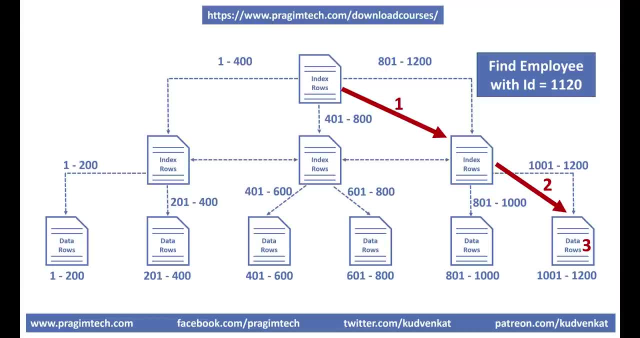 by employee id, SQL server can easily and quickly find the data we are looking for. But what if we search by employee name? At the moment there is no index on the name column, So there is no easy way for SQL server to find the data we are looking for. SQL server. 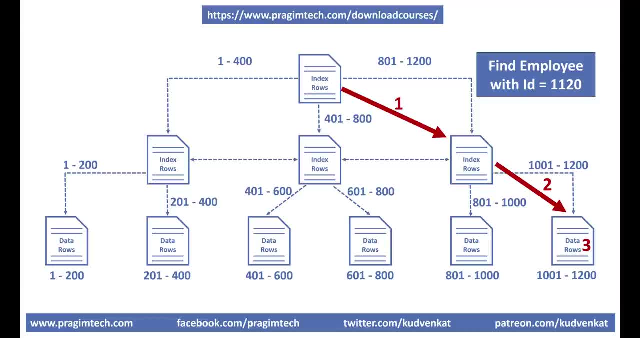 has to read every record in the table, which is extremely inefficient from performance standpoint. That's when we create a non-clustered index on the name column. In our next video in this series, we'll discuss how the index and table data is physically. 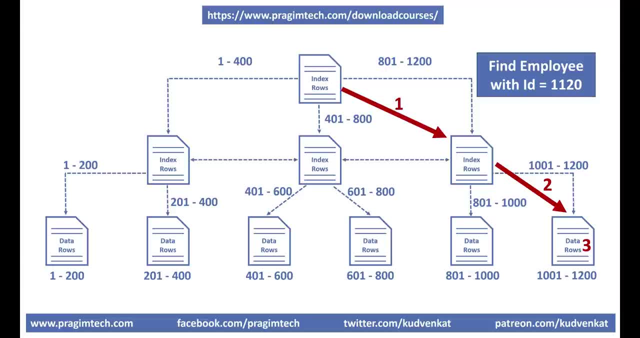 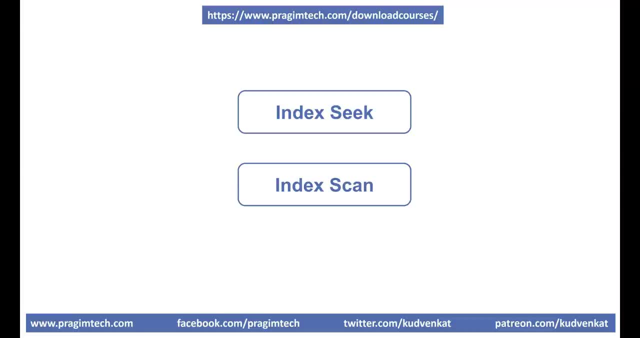 stored when we have both a non-clustered index and a clustered index. We'll also discuss index seek and index scan. Understanding these two concepts is very important, especially when we are tuning SQL queries for better performance. We'll see all these practically in action in our next video. 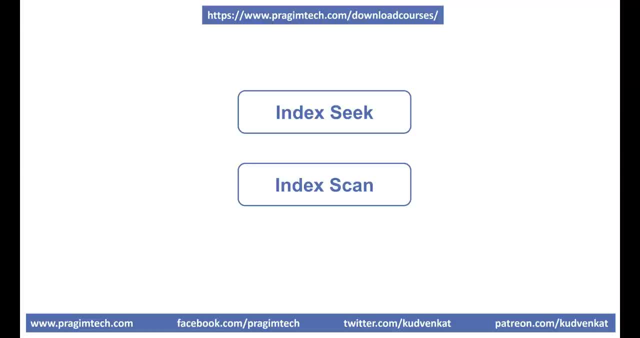 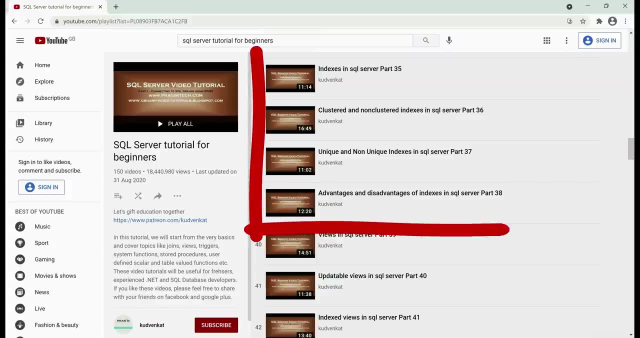 So please stay tuned Before we wrap up. if you are new to SQL server indexes, we have already discussed them in detail in our SQL server tutorial for beginners course. Please check out the videos from parts 35 to 38.. I'll include the link to this course in the description of. 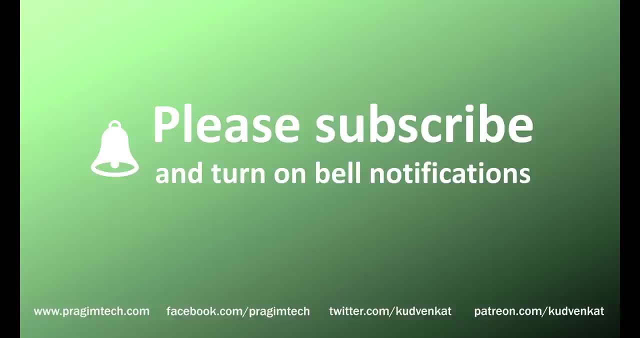 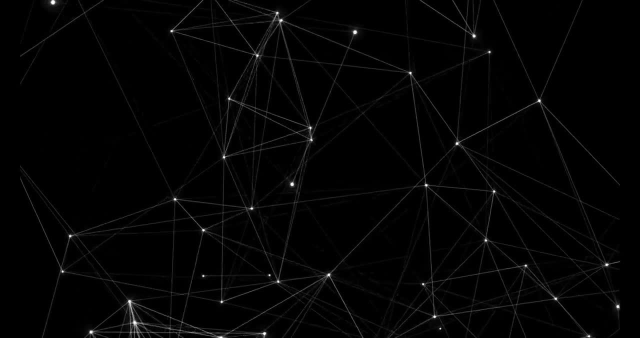 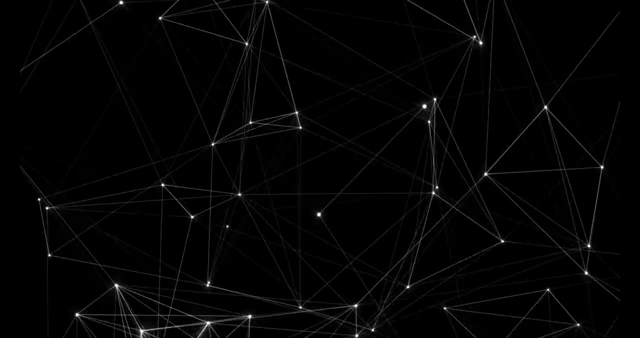 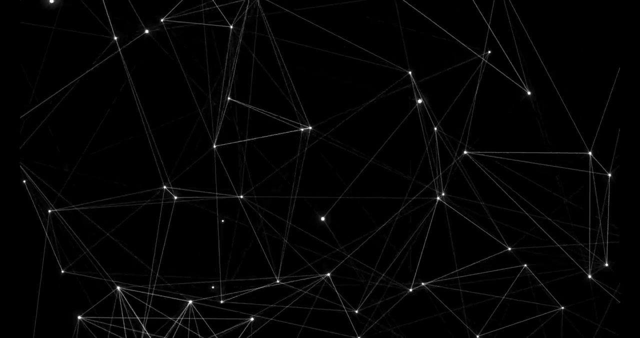 this video. I hope you found this video useful. That's it in this video and thank you for listening. I'll see you in the next video.